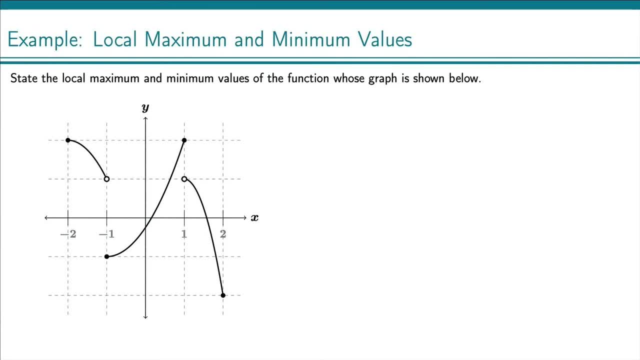 State the local maximum and minimum values of the function whose graph is shown below. Now, when determining local maximum and minimum values, we are not going to ever include the endpoints, like the far left and the far right, And so, like this point right here on the far left, 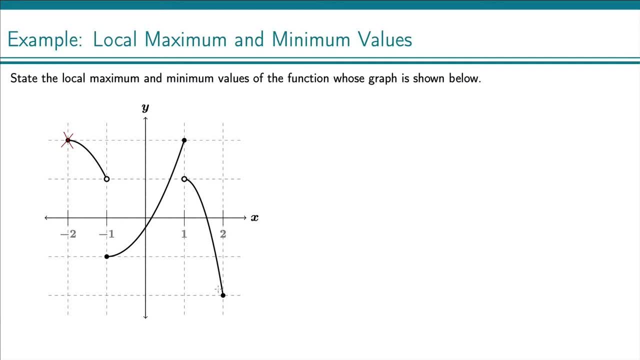 of our domain. we're not even going to consider that. And this point on the far right we're not going to consider. We are only going to consider values between those. So we're looking for points that are higher than all the points around it or lower than all the points around it. So, as we 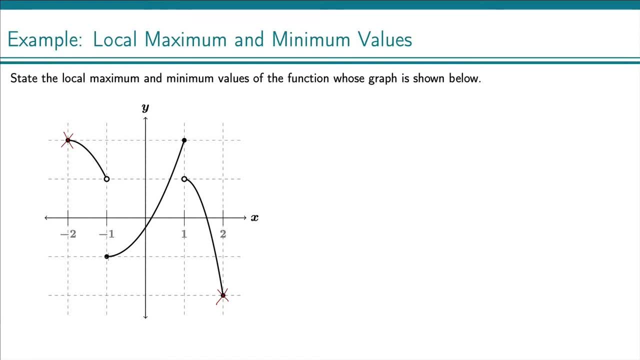 move through our curve here. anytime you've got a jump discontinuity, you're going to want to look at that value and see what's happening to the function there. Here this is the function value and we see that it is lower than the function to the right and lower than the function to the left. 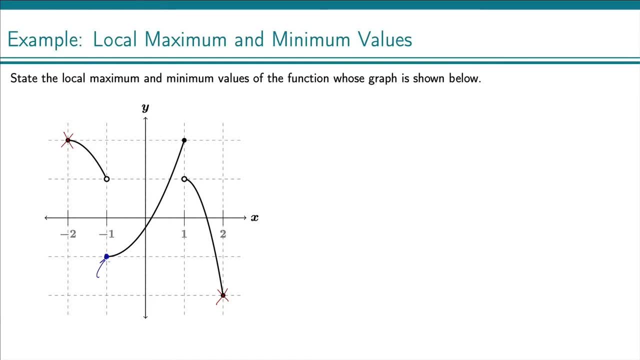 Okay, so this point right here is going to be a local minimum And as we continue, we have here another jump: discontinuity. And this point right here is higher than the points on the left and higher than the points on the right, And so this: 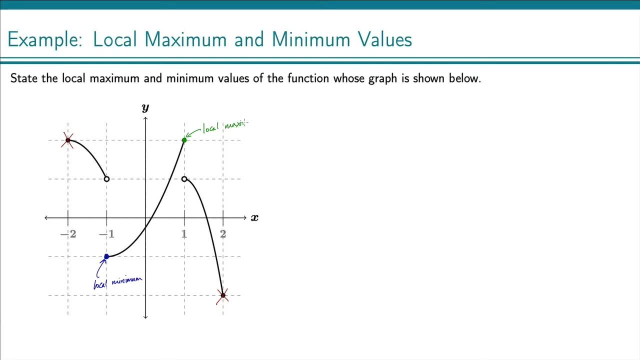 is going to be a local maximum. Now to actually indicate, to specify what the local maximum and minimum values are, we are going to state that the local minimum value is we've got a negative one right here, All right, so that right, there is a negative one. So the y value that's negative one, And it occurs. 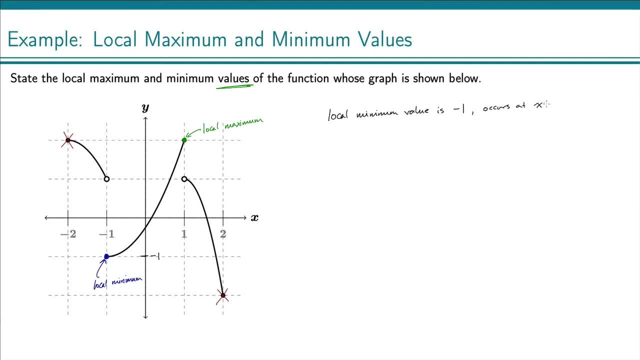 at the x value negative one, this negative one right here. And then for our local maximum. local maximum value is at this point here the y value right. there is two And it occurs at the x value positive one. So those are our only two local maximum or minimum values.